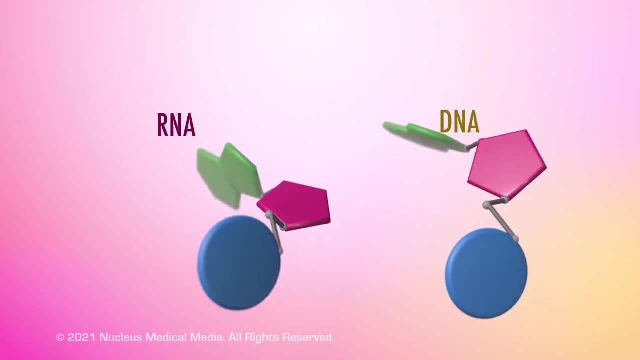 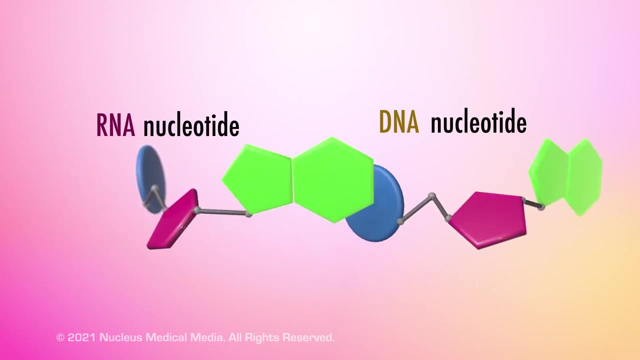 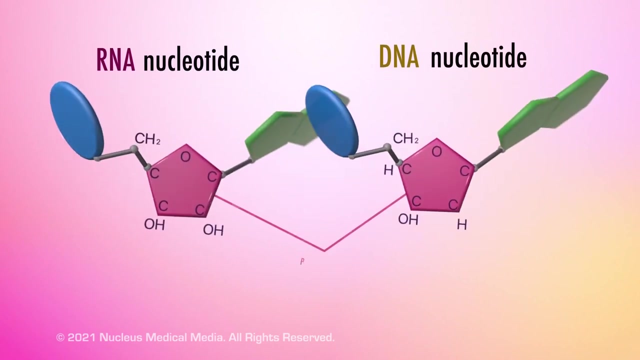 Well, both DNA and RNA are made up of monomers called nucleotides. All nucleotides contain three compounds. The first compound is a phosphate group, which contains phosphorus. The second compound is a five-carbon sugar. All five-carbon sugars can be called a pentose. 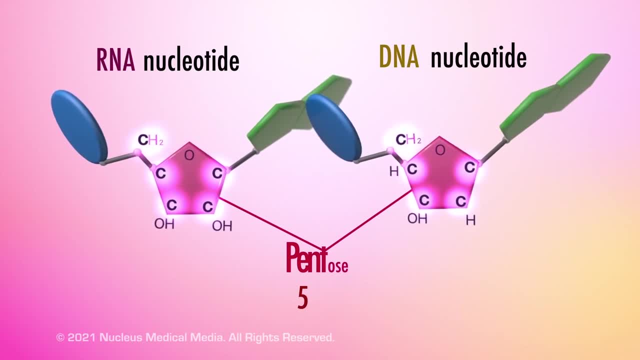 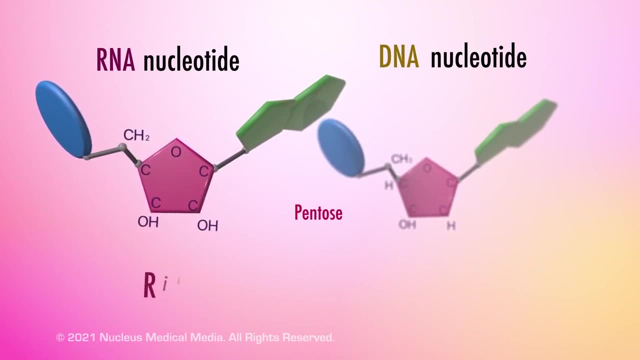 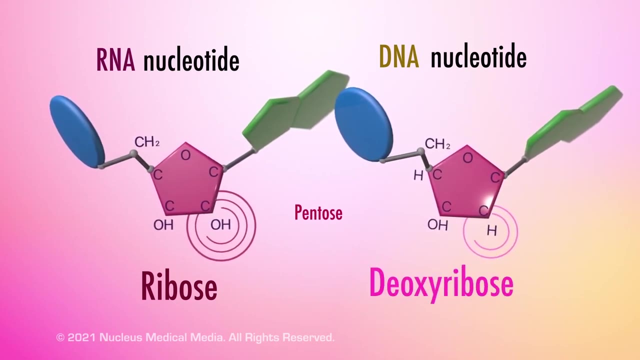 A good way to remember this is that pent means five and the suffix-ose means sugar. The specific pentose sugar in RNA is called ribose. The pentose sugar in DNA has one less oxygen than ribose in RNA, which leads to its name. 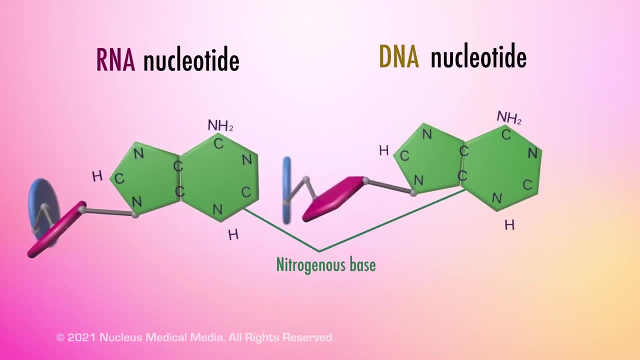 deoxyribose. The third compound in a nucleic acid nucleotide is a weak nucleotide. It is called ribose. The third compound in a nucleic acid nucleotide is a weak nucleotide base that always contains nitrogen. For this reason, this compound is referred to as a 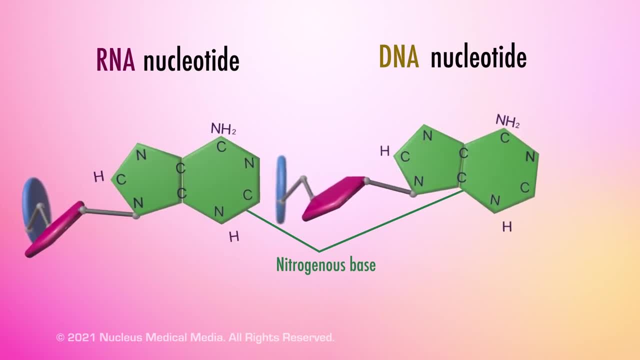 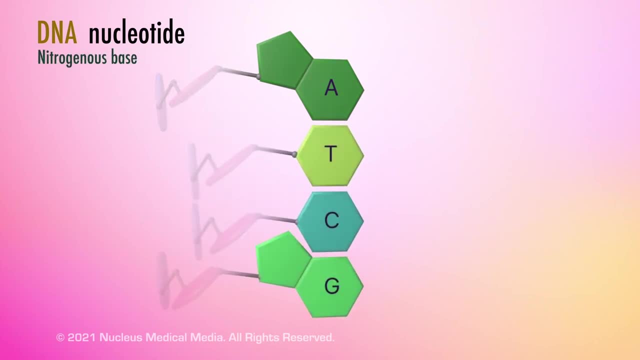 nitrogenous base. The nucleotides in DNA contain one of four possible nitrogenous bases. They are called adenine, thymine, cytosine or guanine. These bases are usually abbreviated as A, T, C and G. Similarly, the nucleotides in RNA also contain: 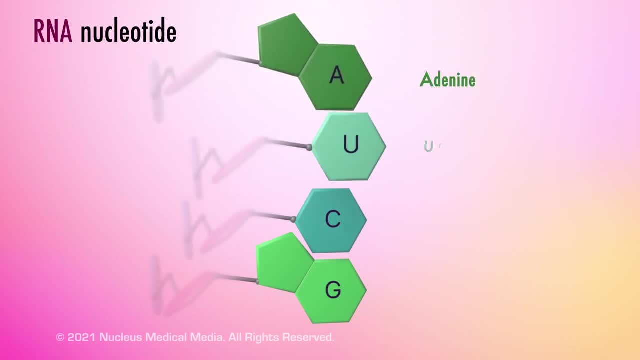 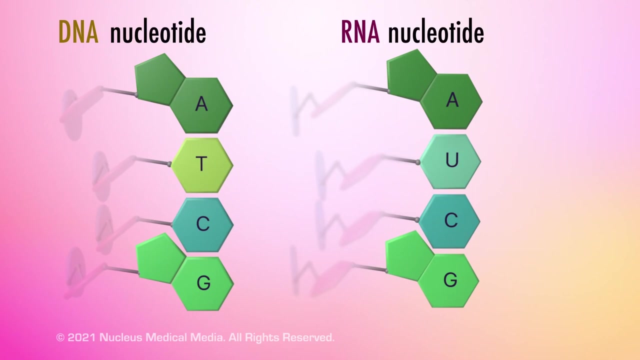 one of four nitrogenous bases: adenine, uracil, cytosine or guanine. They are abbreviated as A, U, C and G. Notice that both DNA and RNA have adenine, cytosine and guanine, but only DNA has thymine, and only 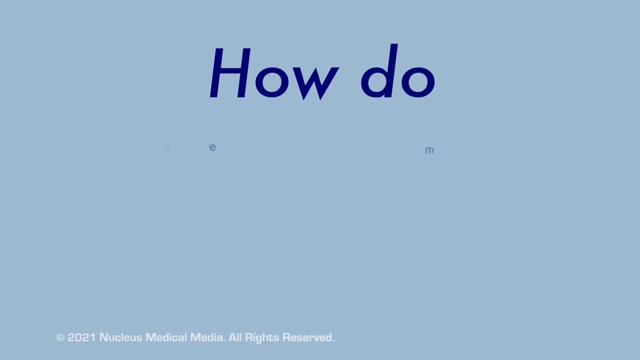 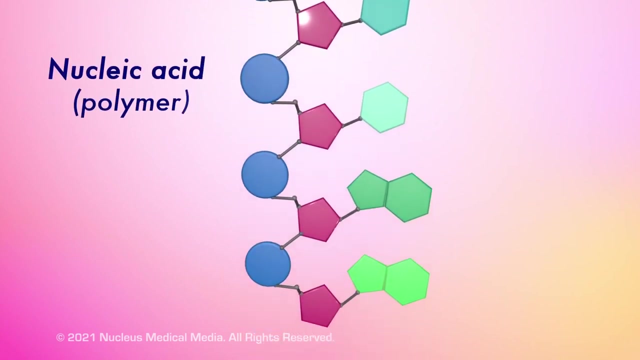 RNA has thymine, RNA has uracil. So how do nucleotide monomers assemble into nucleic acids? Well, the phosphate group in one nucleotide bonds with the pentose sugar in another nucleotide. The assembled string of nucleotides forms a nucleic acid polymer, Even though both RNA 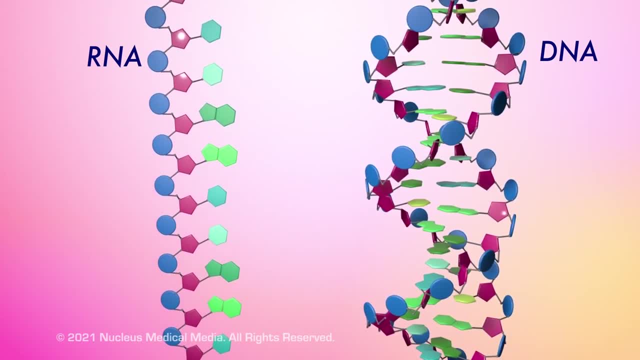 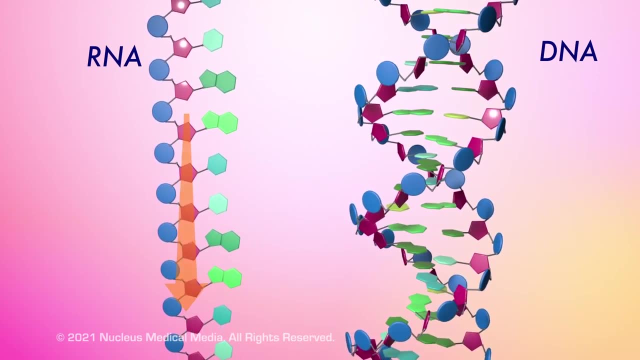 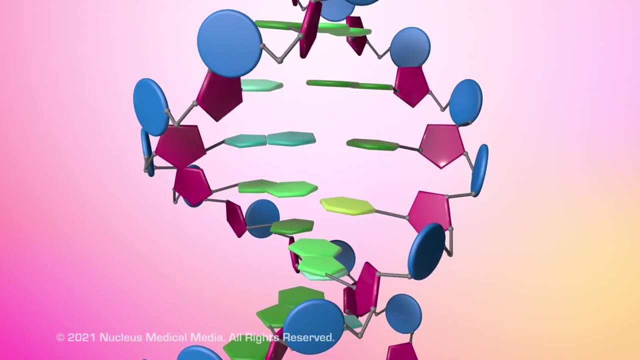 and DNA have alternating sugar and phosphate groups. there are differences in their overall structure. For example, RNA is a single-stranded nucleic acid, while DNA is a double-stranded nucleic acid. The two strands in DNA are linked by a hydrogen bond that connects the nitrogenous